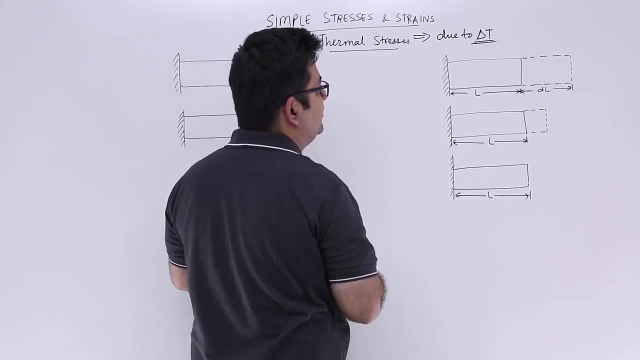 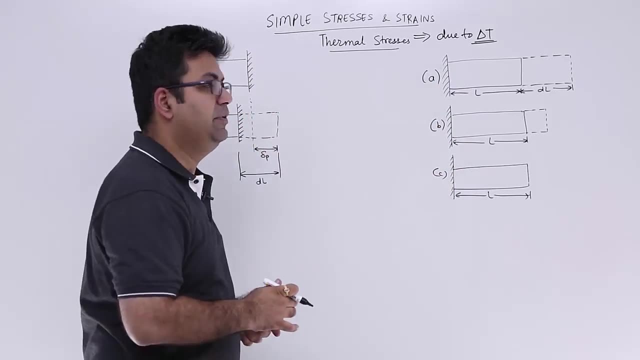 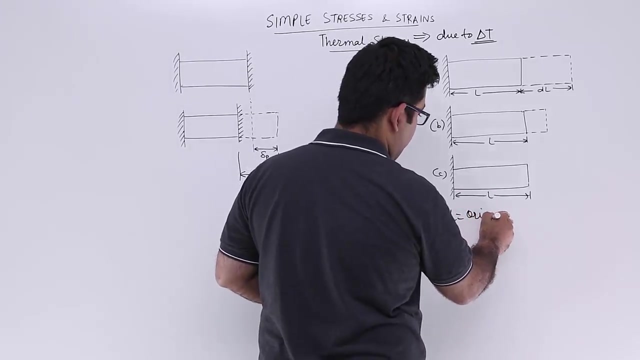 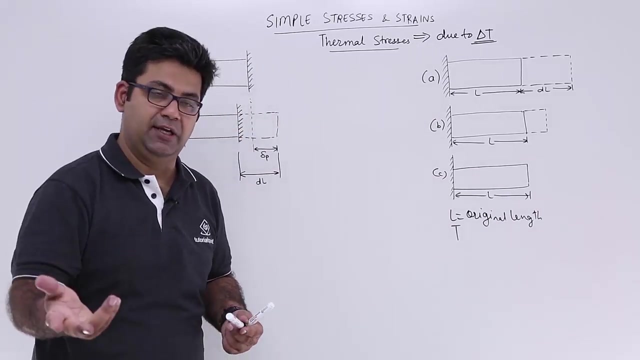 When a body, let us say this is the figure, So I will name these figures as figure A, figure B and figure C. Okay, Some data to remember. that is, let us say capital L is the original length, Okay, And let us say capital T is the change in the temperature. So this is the temperature change. It might be heating, it might be cooling. 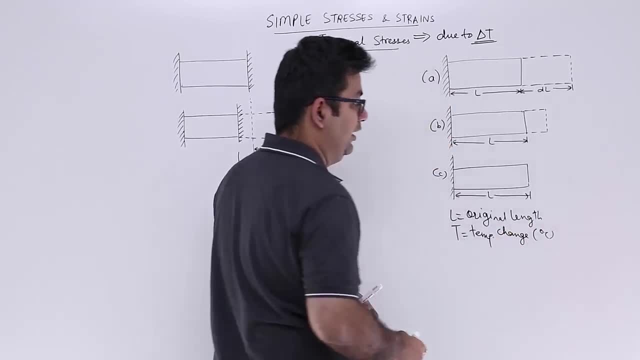 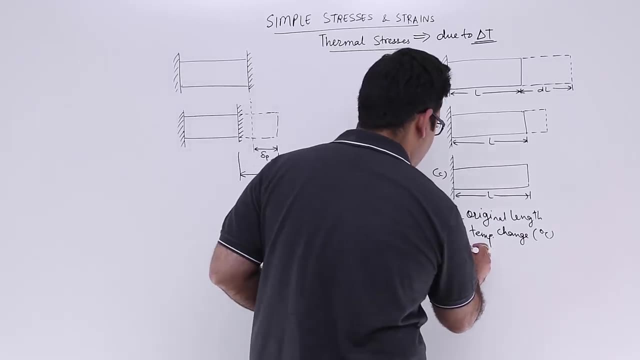 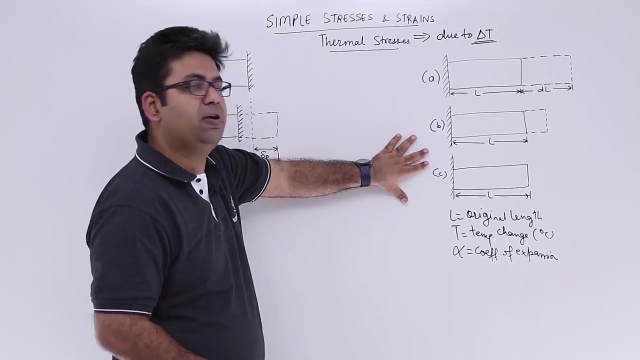 Okay, Let us say this is the degree Celsius. You will have one more value, which is alpha. Alpha is the coefficient of linear expansion, of the material Coefficient of expansion. Okay, Now what happens is: let us right now look at figure number A. Let's forget about figure B and C. At figure A, what is happening? 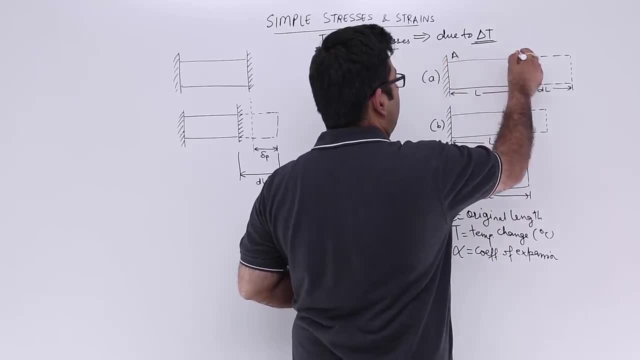 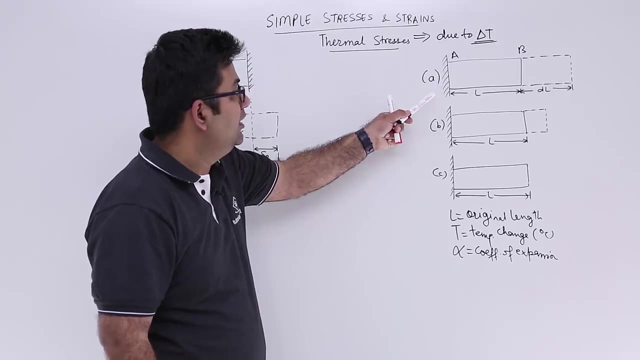 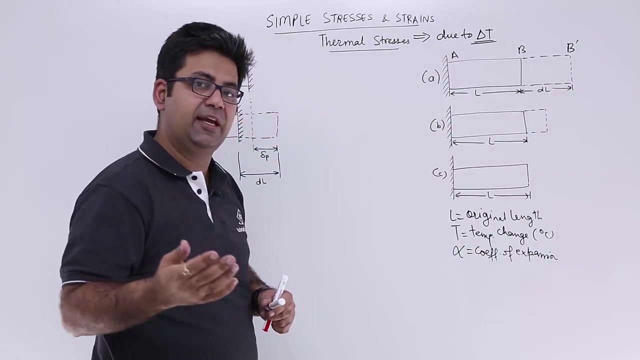 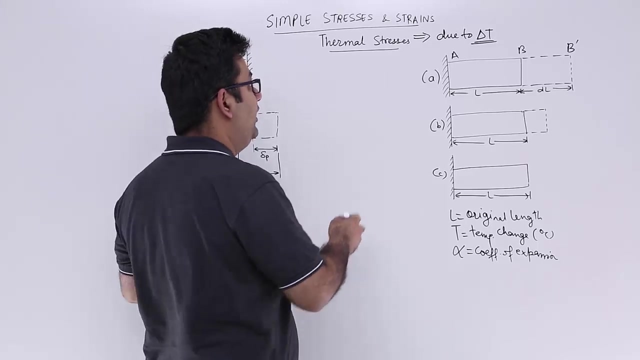 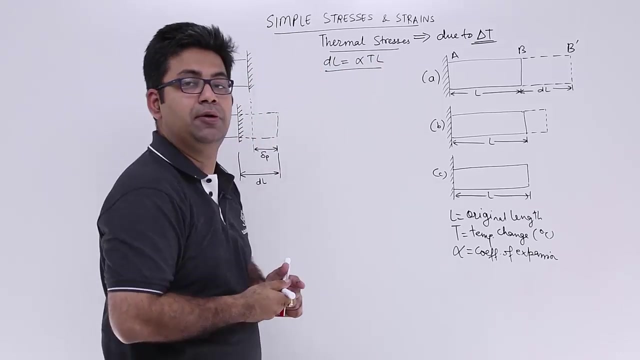 There is no restriction For the material to expand. So when you heat this body at figure A position, So in the condition of figure A, when you heat the body, point B goes to point B dash. So this indicates a free expansion and the length increases from L to DL, Where DL is equal to alpha T, into L. So this is the elongation. 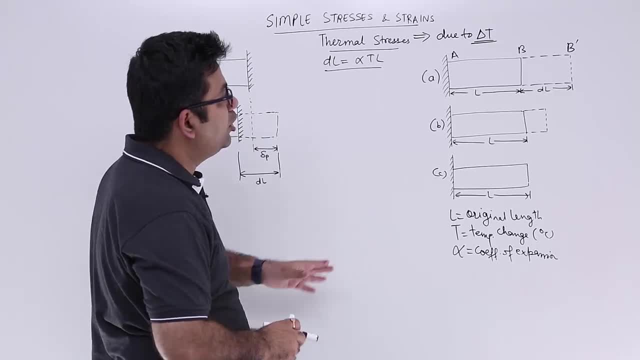 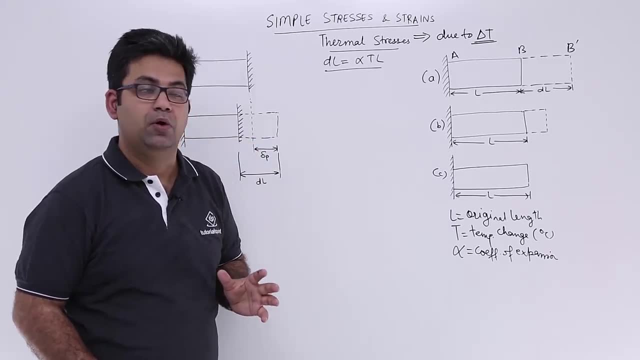 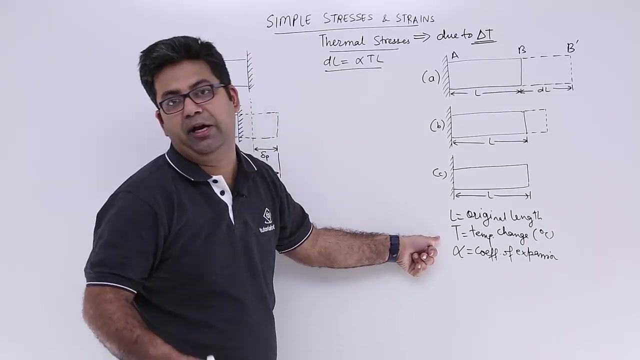 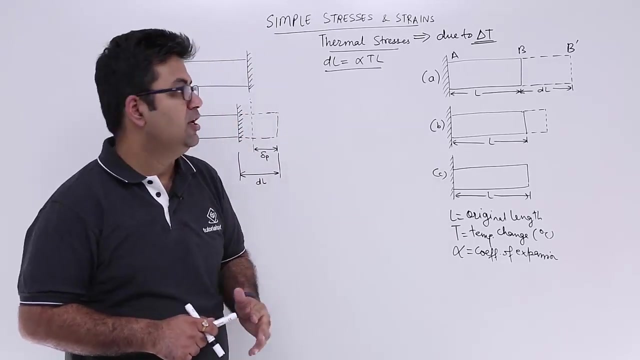 Okay, And let us say we are heating the material. This is the elongation due to heating the material, when the material is free to expand. Okay, So this is that elongation. Alpha coefficient of linear expansion: T is the temperature change. You can write delta T also And capital L is the original length. Now we come to figure B and figure C. So what do I do now? I start applying a compressive load. 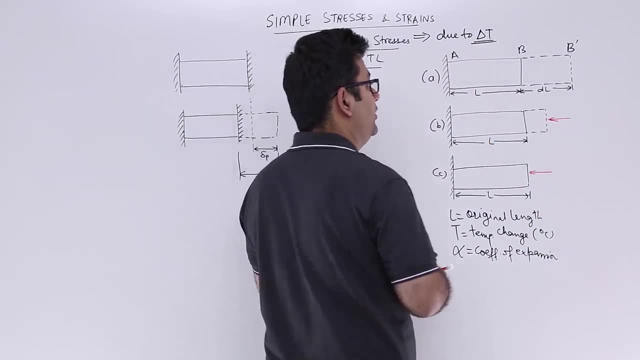 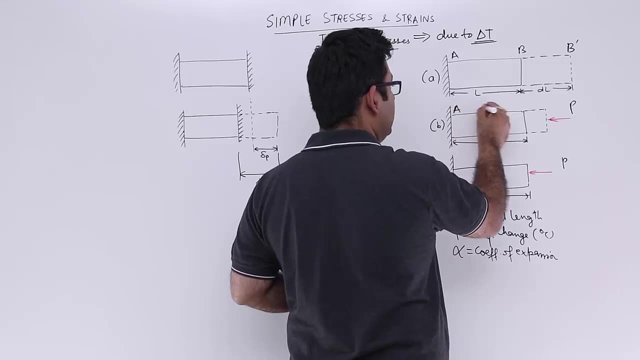 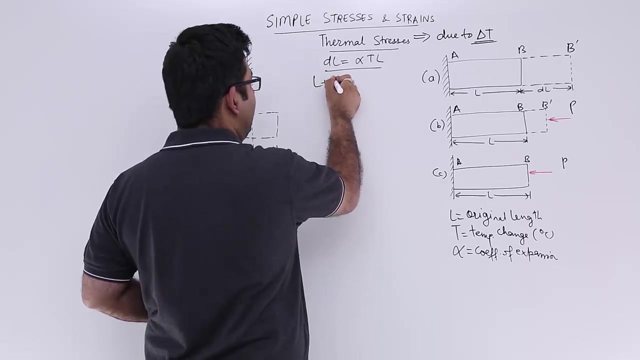 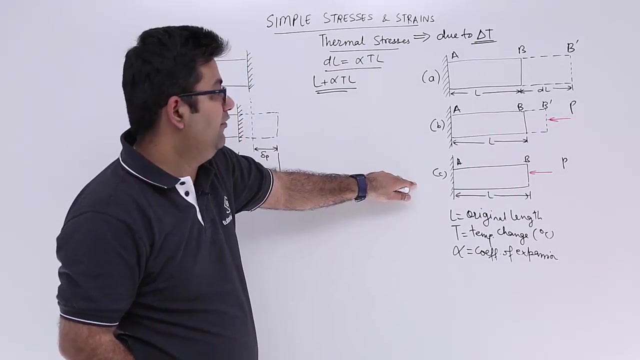 Okay, In the opposite direction. Okay, That is compressive load P. So what happens with this compressive load P is that your length, which was now L plus alpha TL- This was the original length now. So we are going from point A to point B to point C. So now we heat it, It becomes AB to AB dash. Now we start applying a compressive load from the opposite direction. Okay, 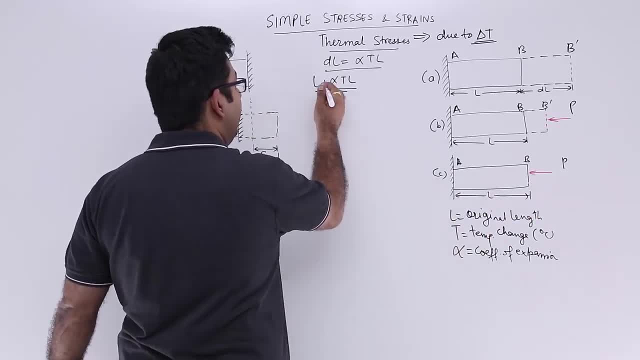 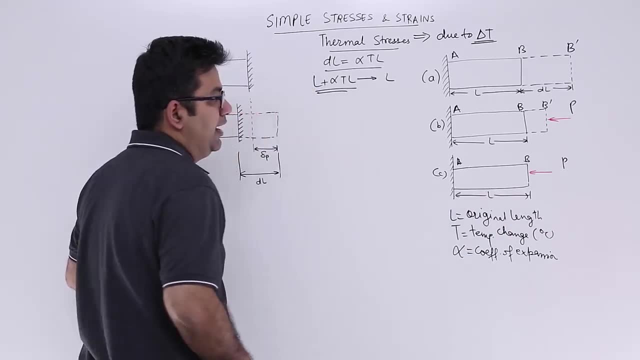 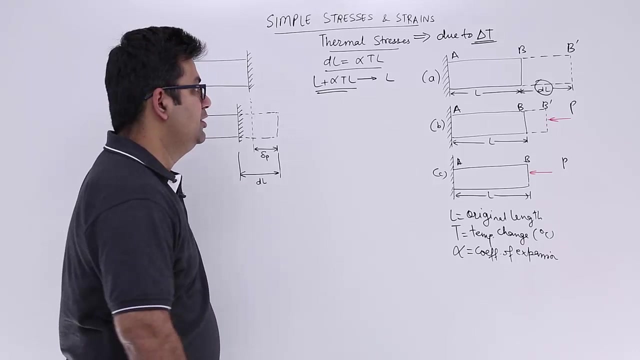 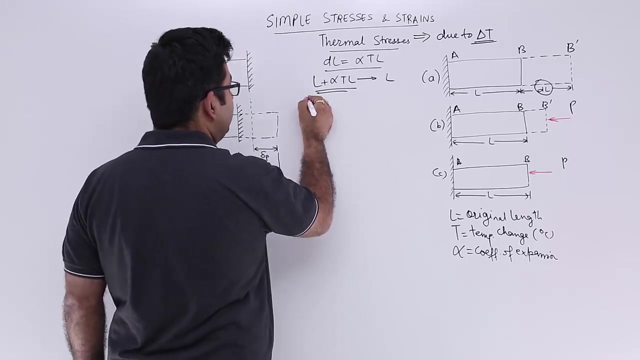 In the other direction, where we are decreasing the length from L plus delta L, alpha TL to L. Now this is compressing and finishing this extension. So this means we are compressing it, Is it right? So there will be some amount of compressive strain in the body. So that compressive strain, I would say EC, is the change in the length. Okay, 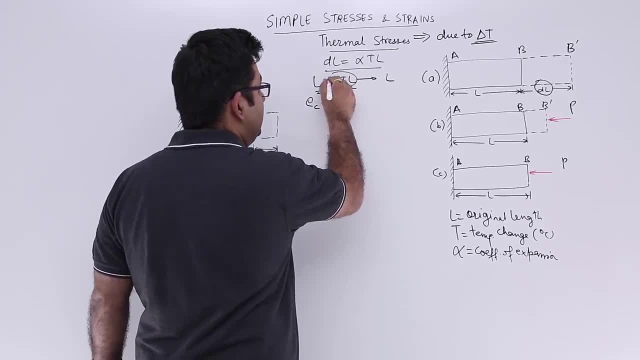 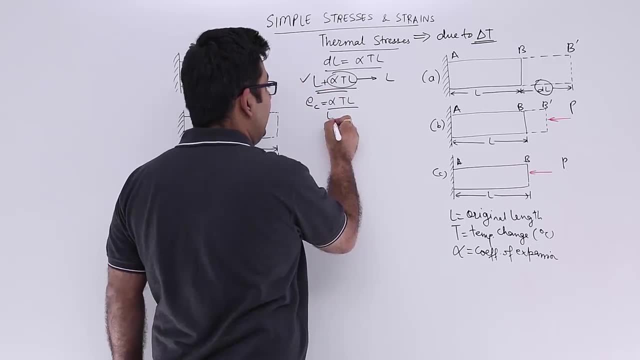 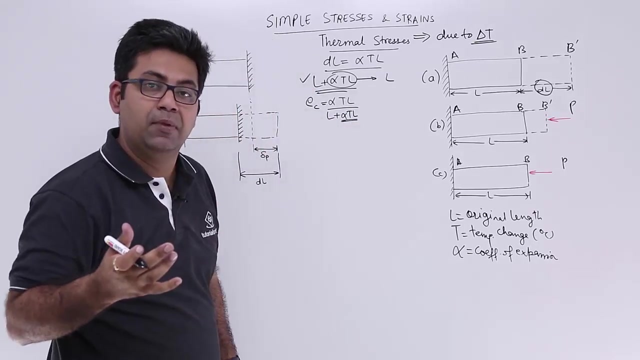 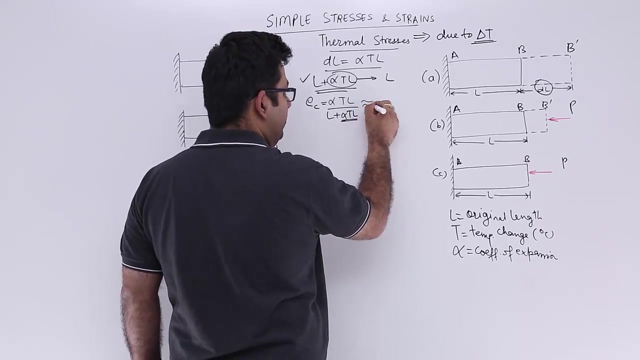 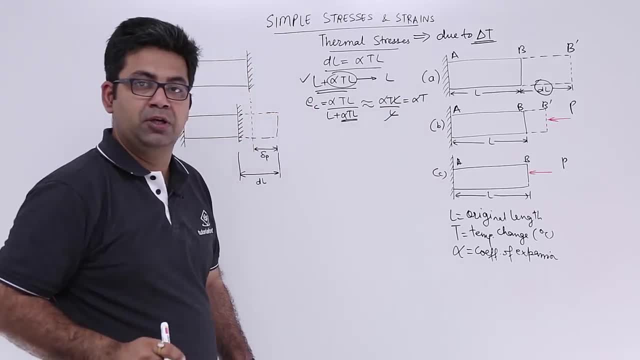 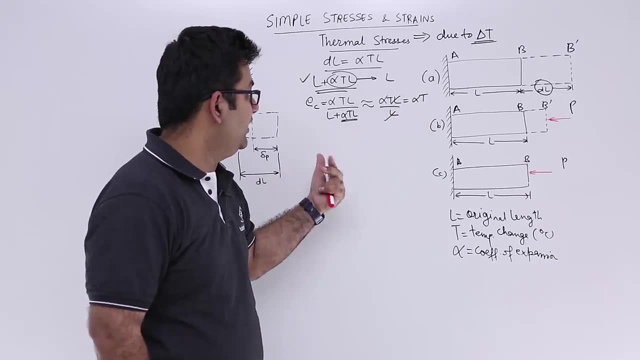 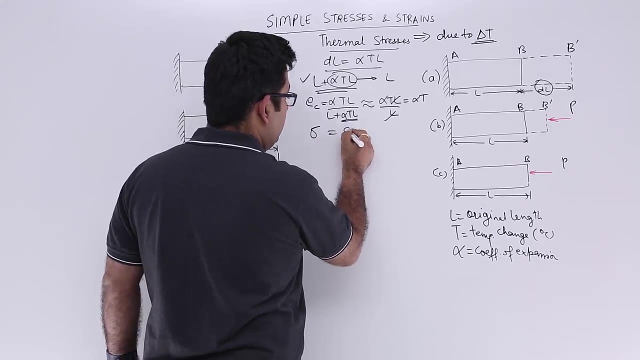 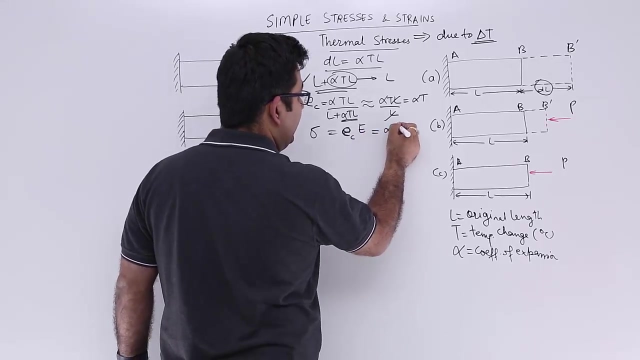 will cancel off and you will get alpha t. so the compressive strain that comes into the body now is alpha t. due to this compressive strain will have a stress and that stress is equal to strain into the young's modulus. now this is equal to alpha into t, into e and 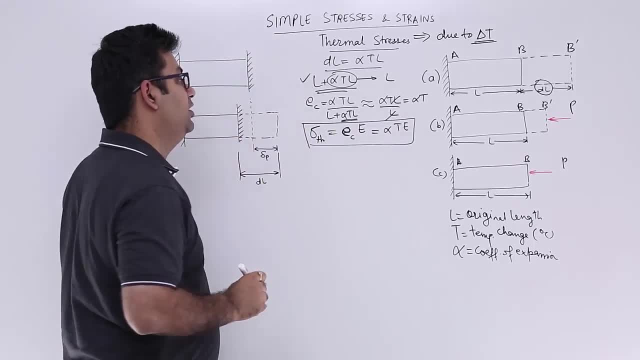 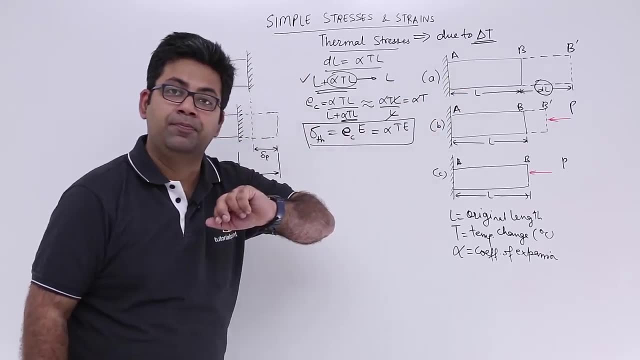 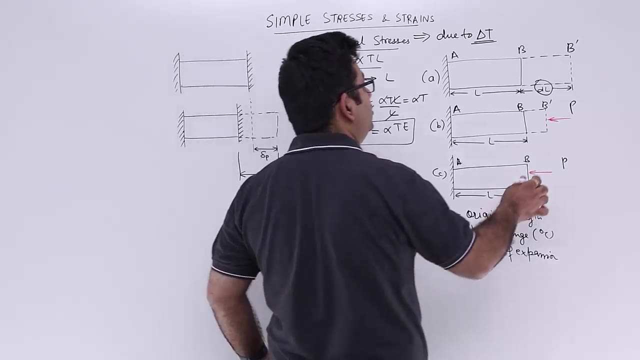 this is what we call the thermal stress. so now we come to a very important conclusion. that is, when the body is free to expand. yes, it will expand due to heating, or it will contract due to cooling, but there will be no stress. so sigma th is zero in this, because there 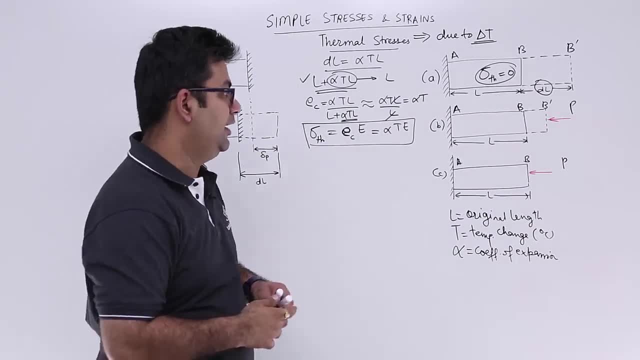 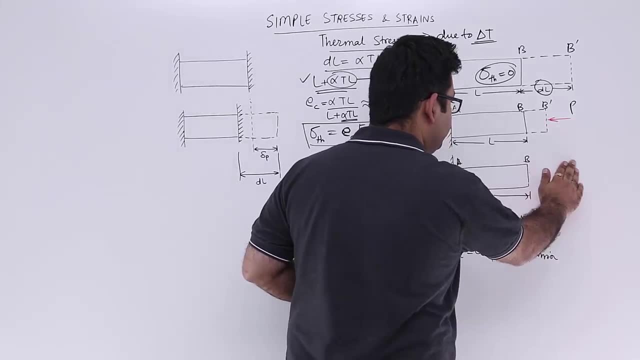 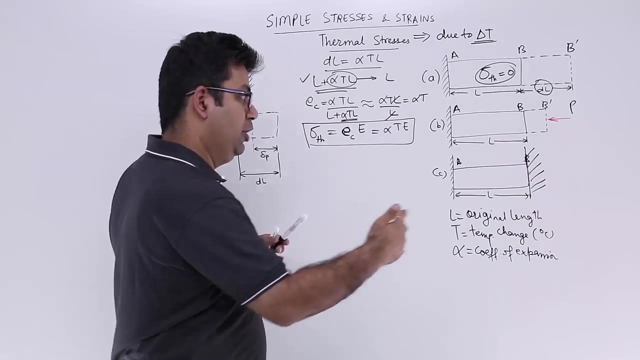 is no restriction, okay. but now let us say we have a load like this: or let's remove this, move the load. for a better understanding, let me put this body between two fixed supports. this body cannot move anywhere. so now you start heating the temperature, now you start. 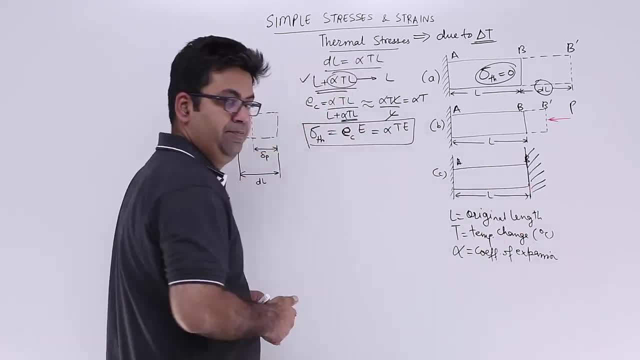 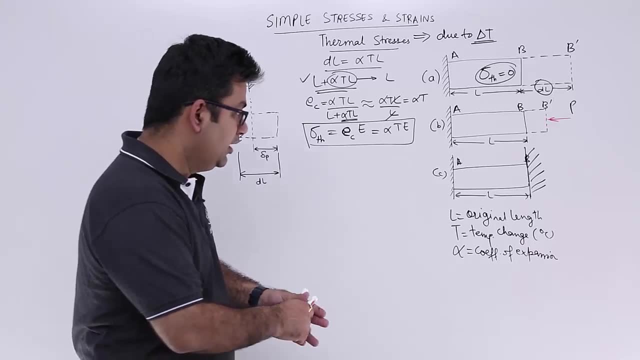 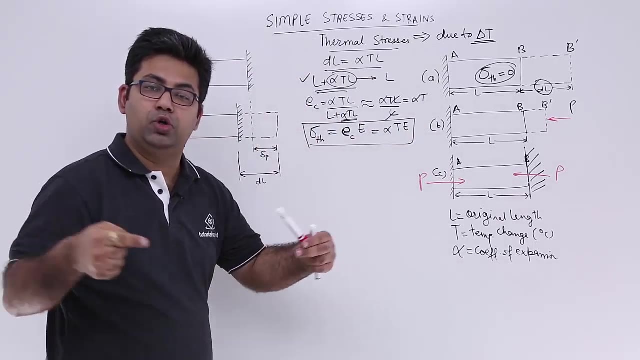 heating the body, it will try to expand, but obviously, but due to these two fixed supports, it cannot move. it cannot move why? because these two supports are producing or are applying a compressive load onto it which is, you know, preventing the body to expand freely and due. 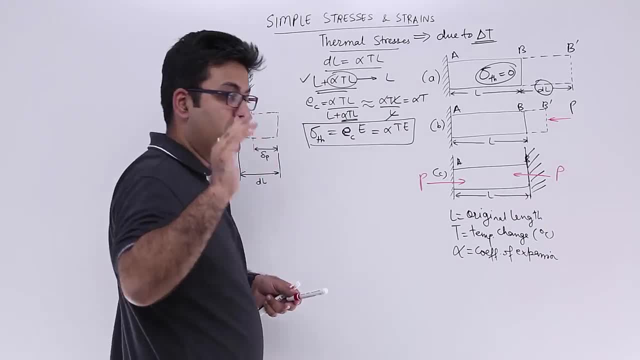 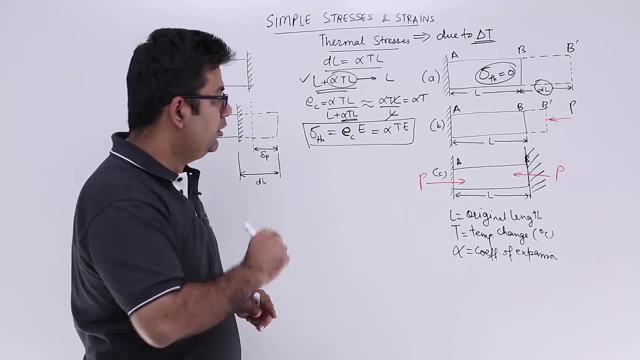 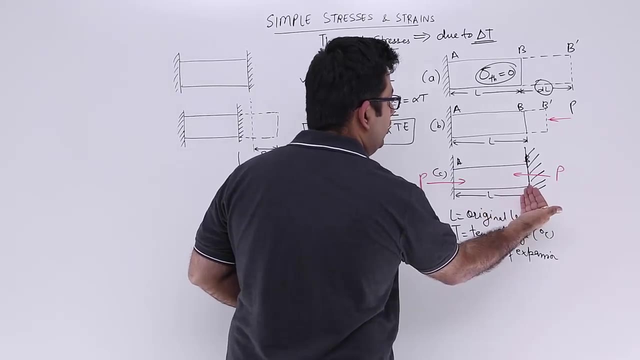 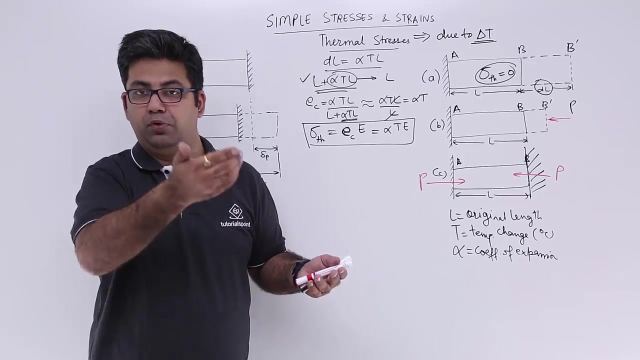 to this compressive axial load, there is a production of thermal stress. okay, so i hope you got this concept. now a very important concept comes into picture. that is, what is support yielding? support yielding means any of the supports it starts to shift it yields. it basically loses its meaning of the support. the support comes out, okay. so 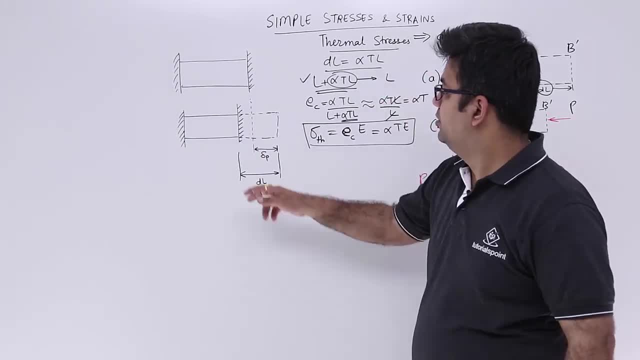 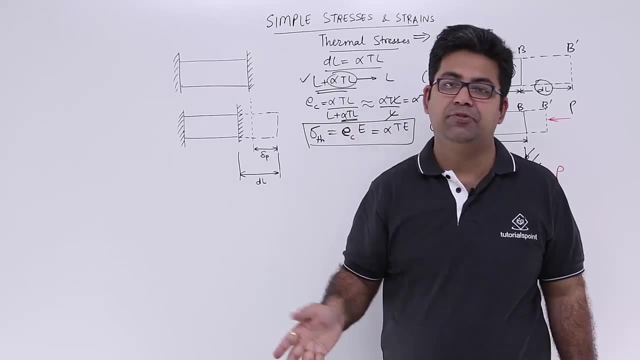 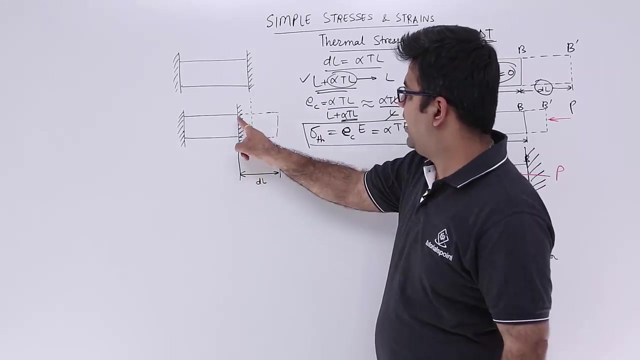 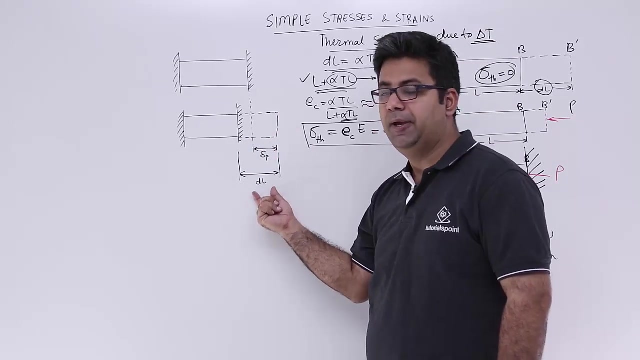 let's come to that figure over here. so this is what you have. this is the body in the two supports. okay, so for a moment, let's forget that there is a support at the center. it is free to expand. so when you heat the body, it will expand till this point, so that this is the total expansion, which is dl. okay now. 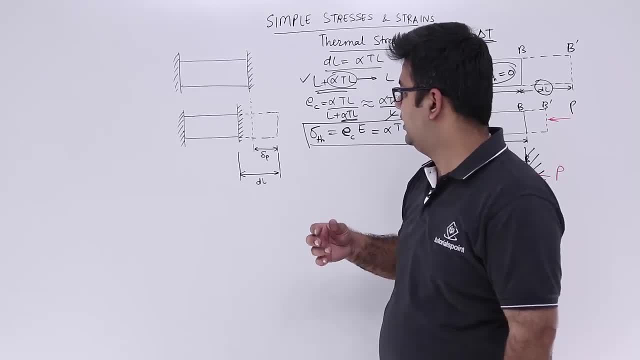 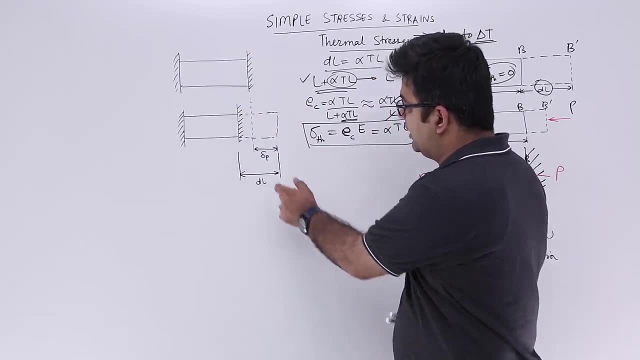 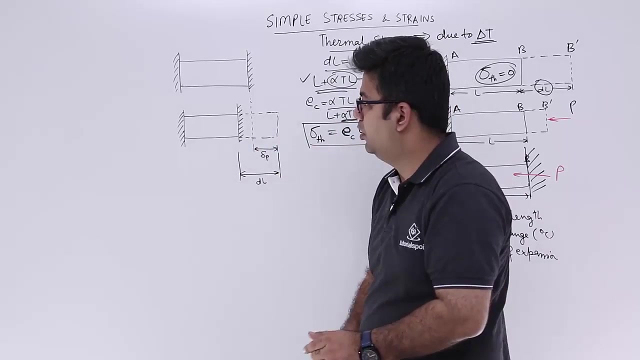 what happens is, let us say, let us say now, let's put it into two supports. so when the support is there, this much, this much will be retraced, this much elongation will be vanished because it has to come back to the support. so this is the 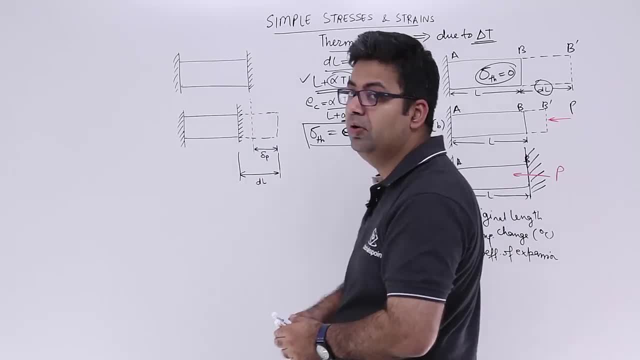 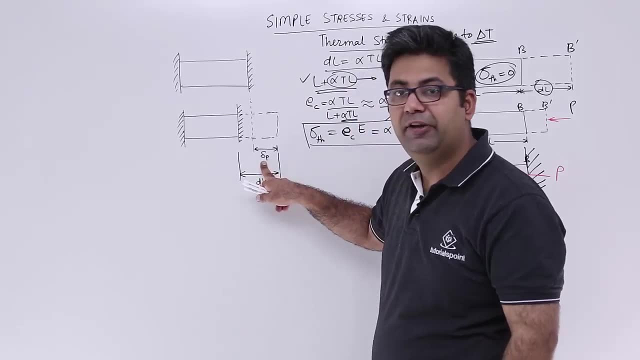 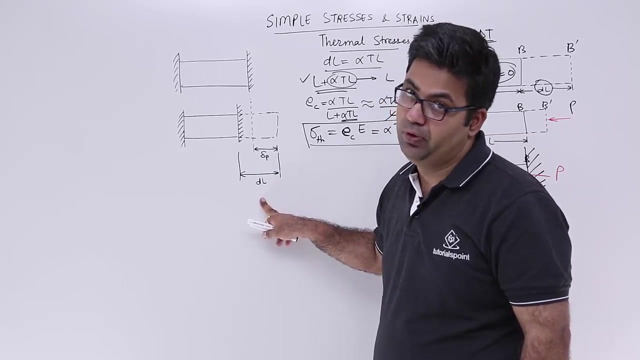 deformation or the contraction which comes into play due to this compression because of the supports. okay, So this is the deformation due to the compressive axle load. This is the elongation which comes into picture when there is no free support or when there is no support to restrict the expansion of the bar. 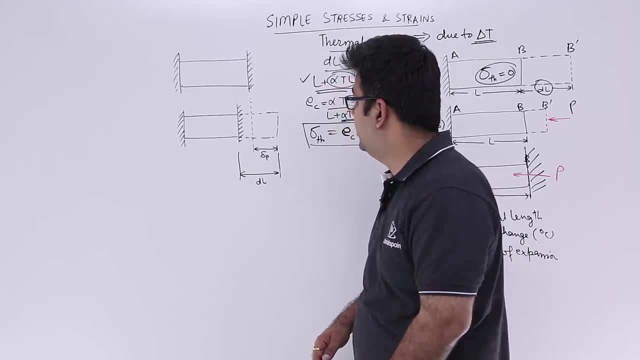 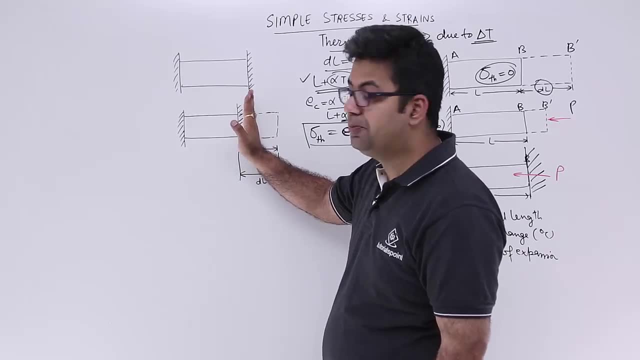 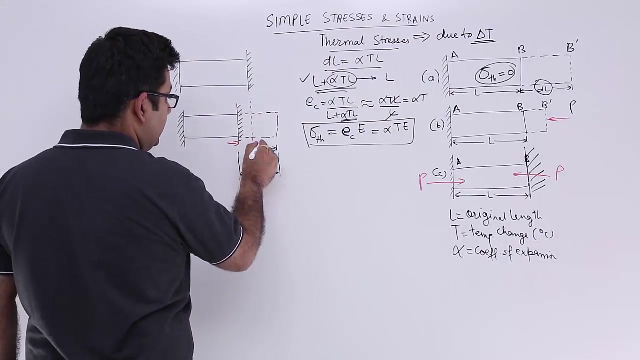 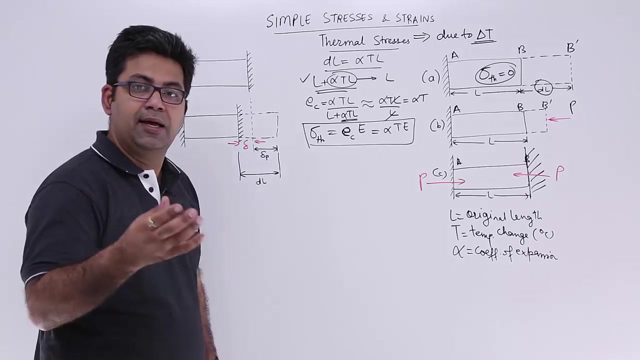 Now what happens is basically due to excessive compressive load generation. this support moves from this point to this point, So this is called support yielding. okay. So let us say: the yielding is delta. the yielding is delta, okay. So what is the actual expansion? 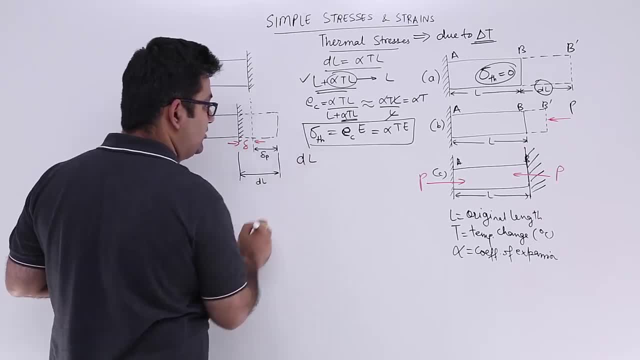 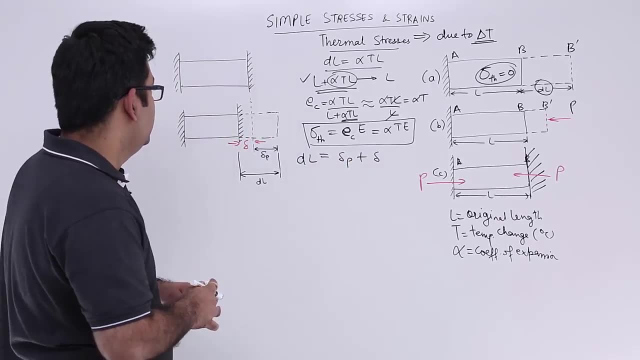 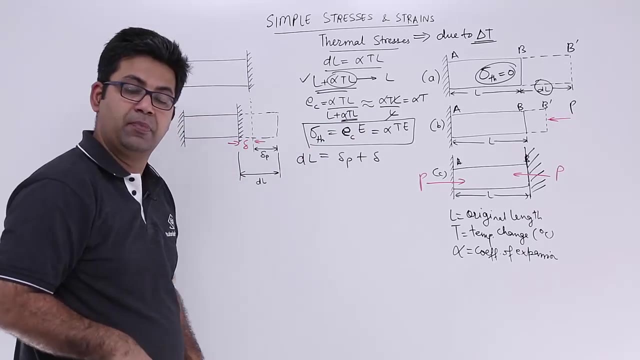 If you look at this, DL, which is due to the free expansion, is basically a sum of delta, P plus delta. I will repeat this. So let us say: this is the support. So if there is no support, it will expand freely. This is the free expansion. Now, if you put a support over here, this much expansion will. 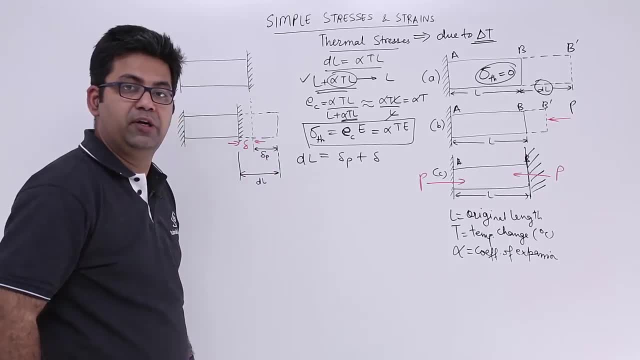 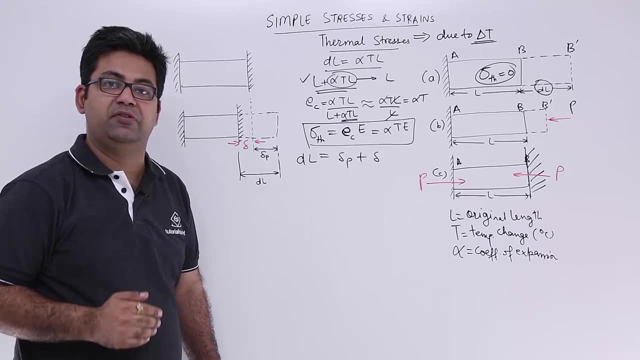 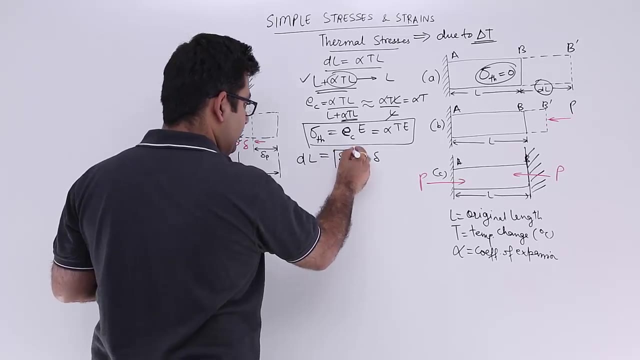 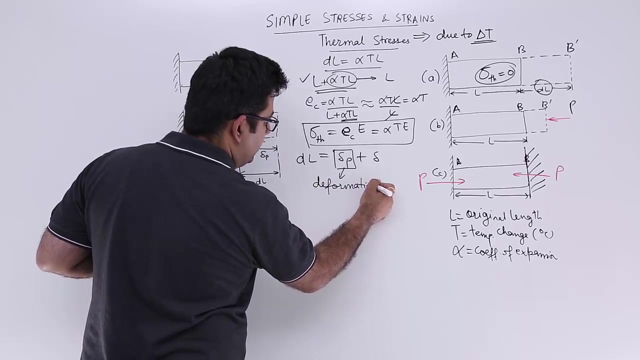 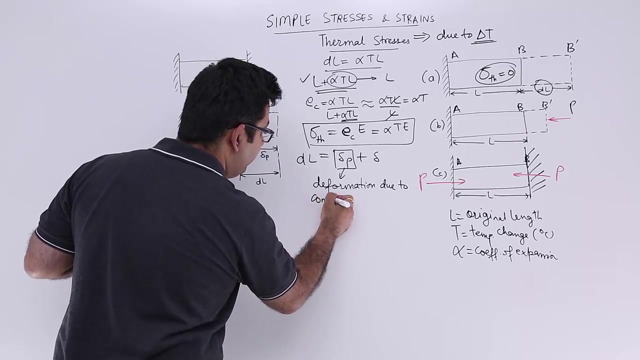 be vanished because it cannot go the whole distance. okay, So now what is happening further is this entire support has moved, So you get the DL is equal to delta D plus delta. okay, So this is basically the deformation, or you can say elongation or contraction. I will just say deformation due to compressive. 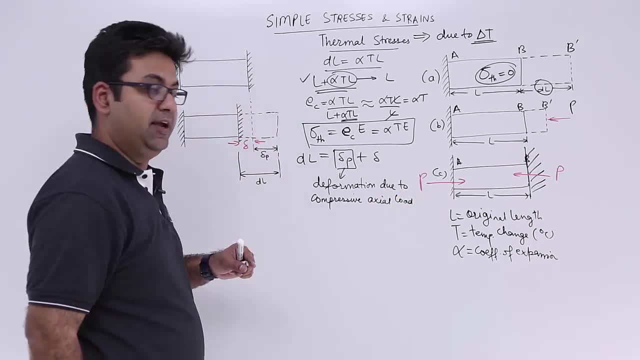 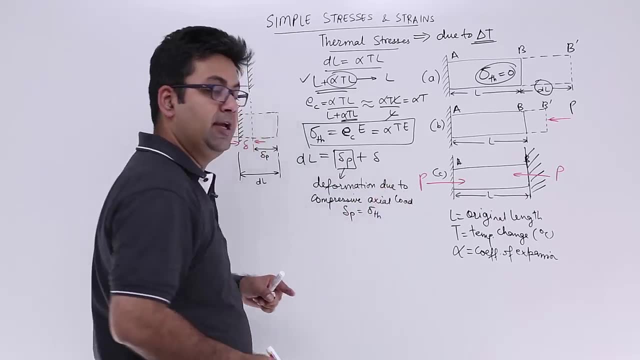 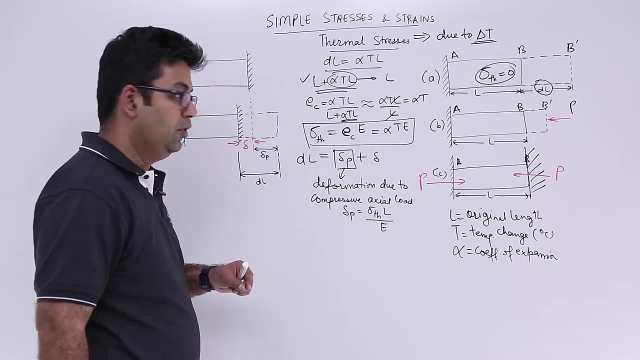 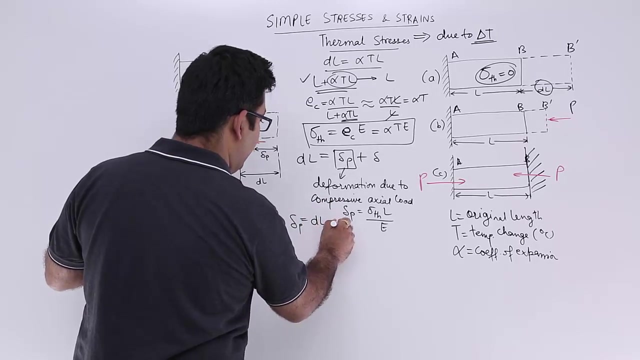 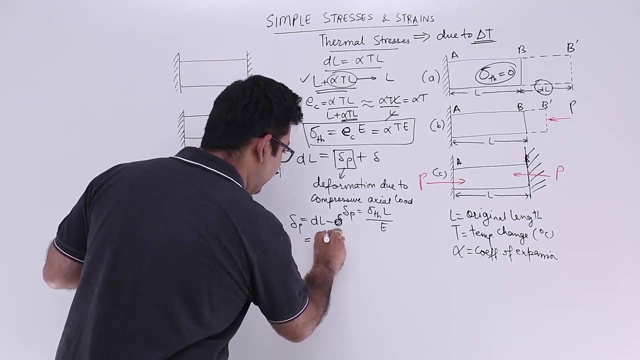 axial load. okay, so this is what we are mostly interested in. so delta p is equal to sigma th, which is the thermal stress- i told you that- into l upon e. okay, so this is what we are interested in. so delta p is equal to dl minus delta. okay, so dl, we know, is alpha tl minus delta. so this: 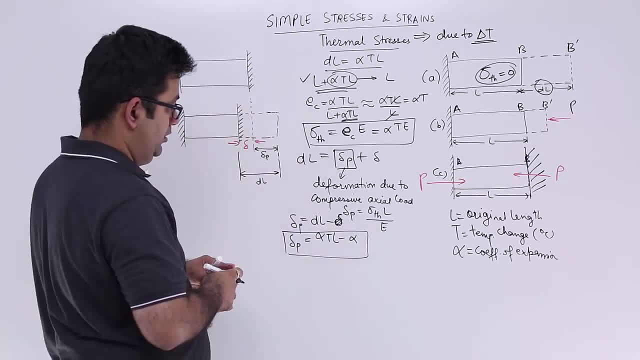 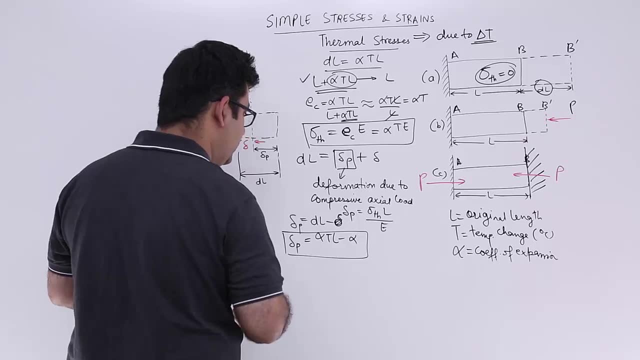 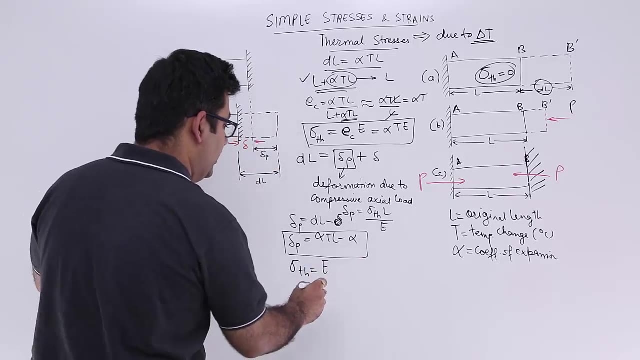 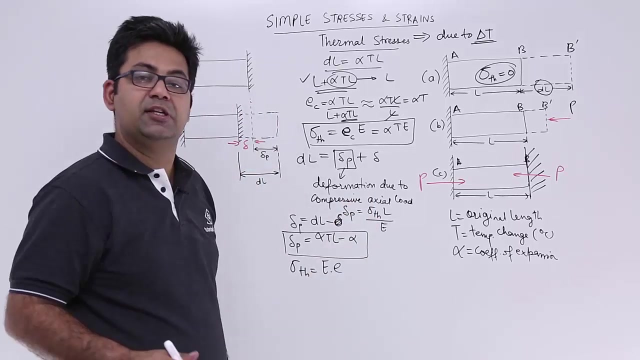 is the- you can say, expression of our interest, right? so if you have to find out the thermal stress due to this, so thermal stress due to this would be equal to e, or i would say this would be e into the strain. now, what is the strain in this case? this is the deformation. 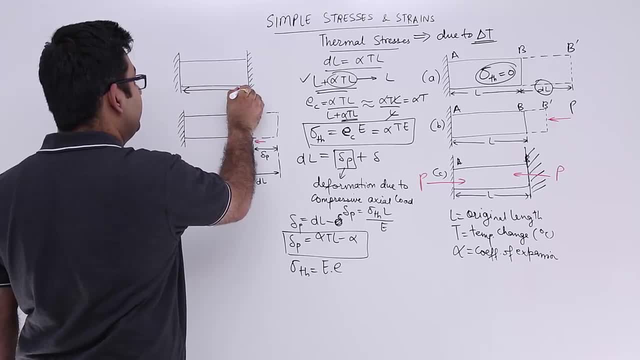 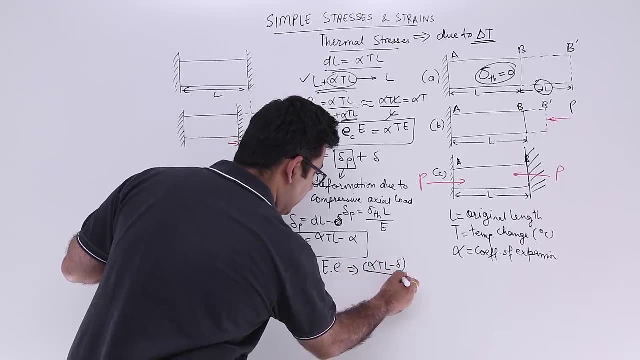 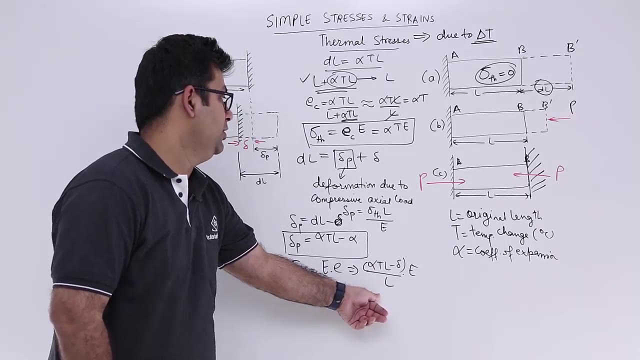 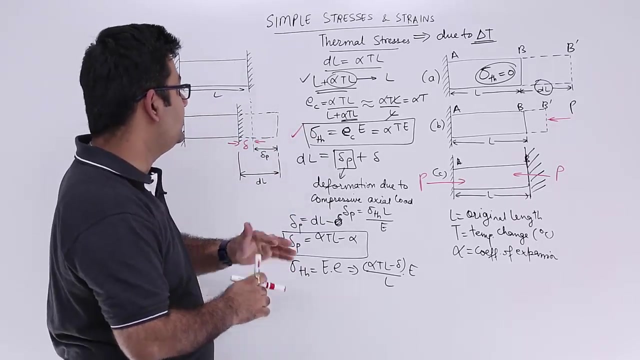 or the, i would say, contraction. the original length was l, so e in this case would be alpha tl minus delta upon l into e. so that is the thermal stress. okay, so if you look at this particular equation over here, this particular equation, this can be said. this equation can be said as the equation.